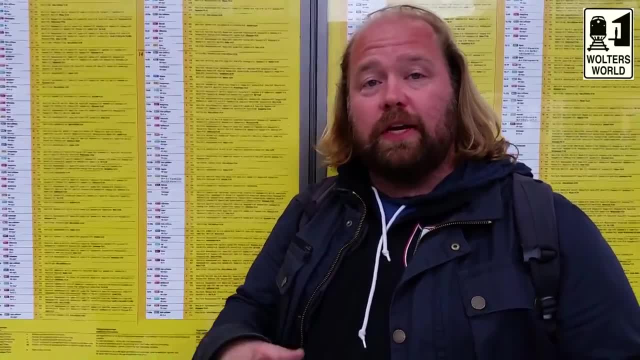 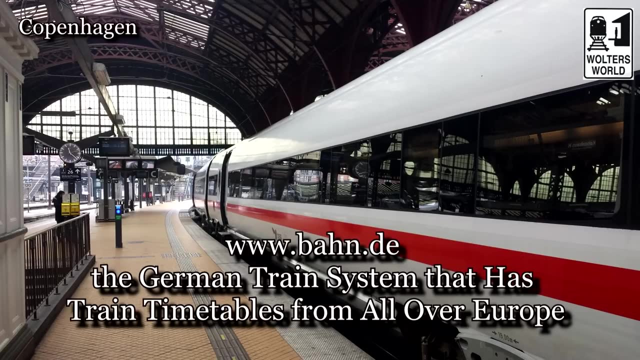 that do go Now. not all trains will show up on these websites, but it'll give you a good idea. I like to use bondde, and on there they have train timetables for all over Europe. Okay, another thing you can do is when you come to the train station. you can either. 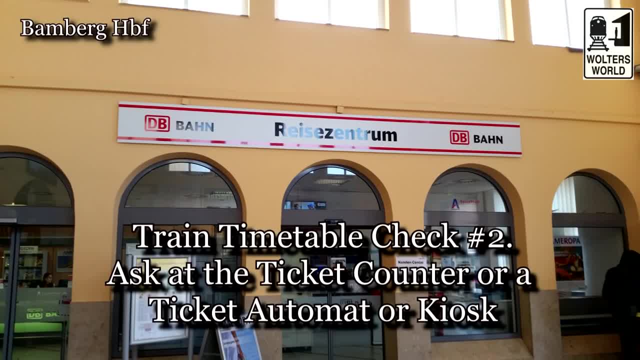 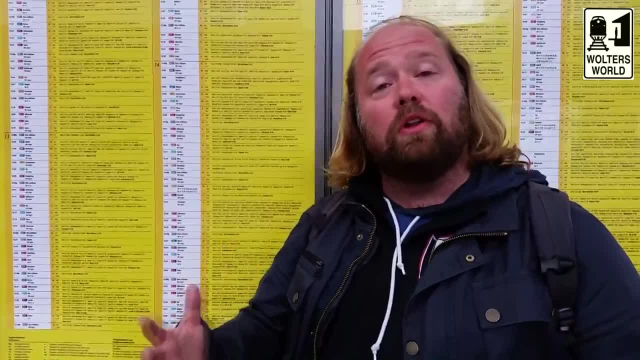 go to the ticket office and ask there, but that takes forever- or use one of the automatic keys. They have them here in Oslo, they have them in Berlin, they have them in London, they have them all over and you can search for train times on there. so you have an idea when. 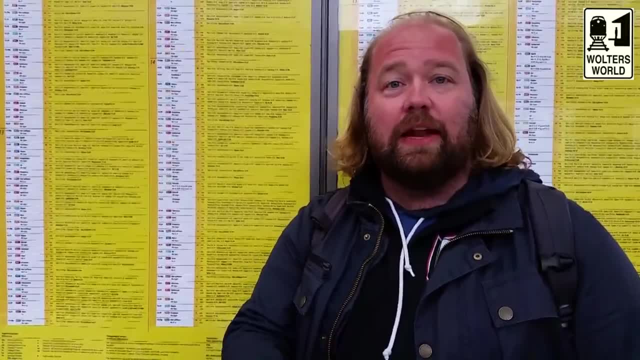 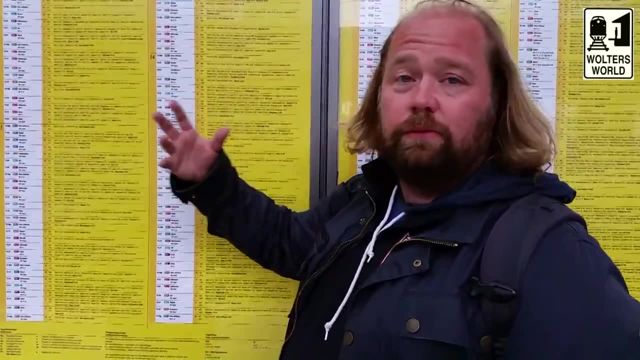 your trains leave when you need to be there or when you're going to get in and things like that, And then they have it the old fashioned way. You have signs like this up on all the train stations, or most of the train stations in Europe, and they'll have either departures. 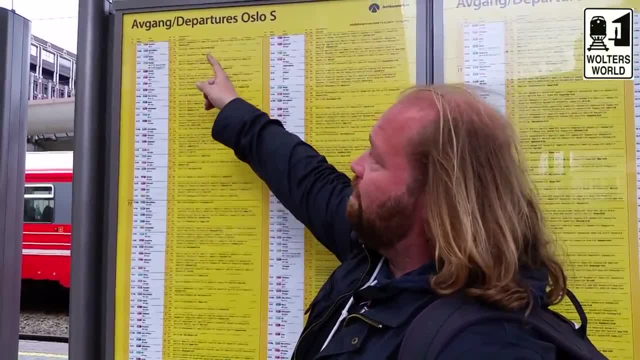 and arrivals. Make sure you look up here Now. up here you see, it says Avgan, but it also says departures. So you know these are the departures from here in Oslo. So what you look on here is it'll tell you the train times. So if you're in Oslo, you're going. 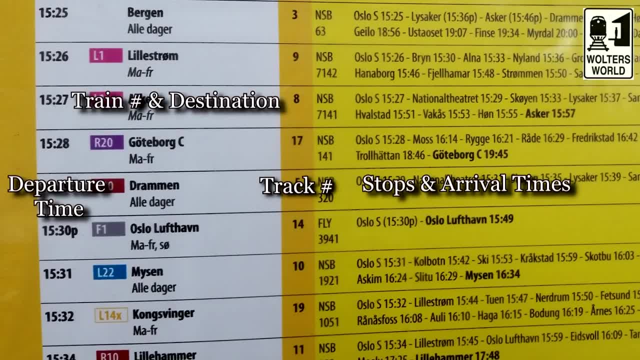 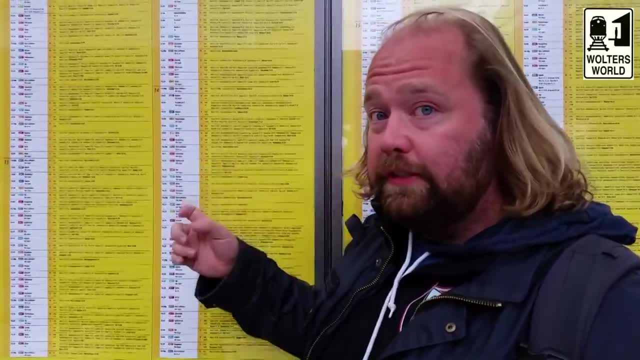 to have the train, the time the train leaves, the number of the train also, where there's some of the destinations that are on the way. Now it might have all the destinations or it might not, but you want to look and see. is my train destination on here? Then, if it, 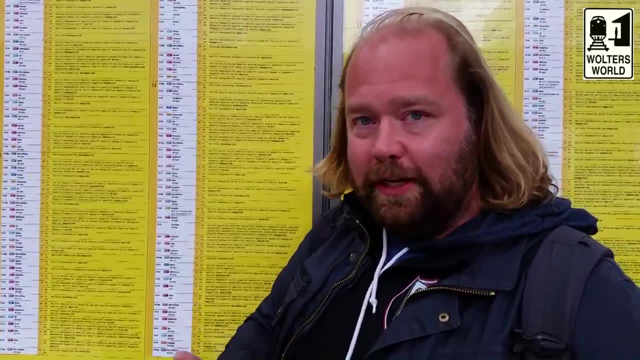 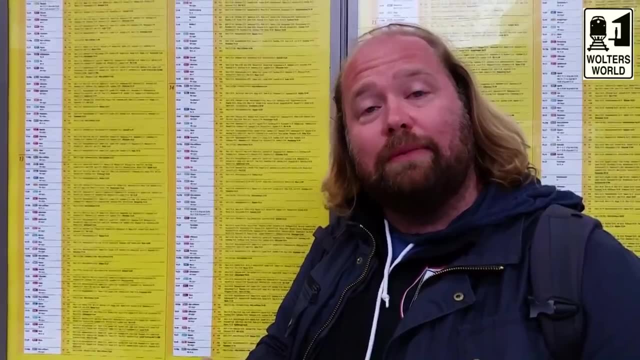 is: look and see some of the other stops. so you know, hey, when should I get ready to get off my train, in case I miss it, okay? So those are kind of like the three kind of ways you can check your train timetables. Obviously, if you've got your phone you can. 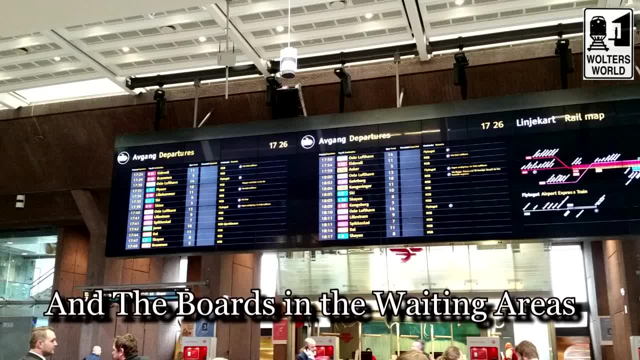 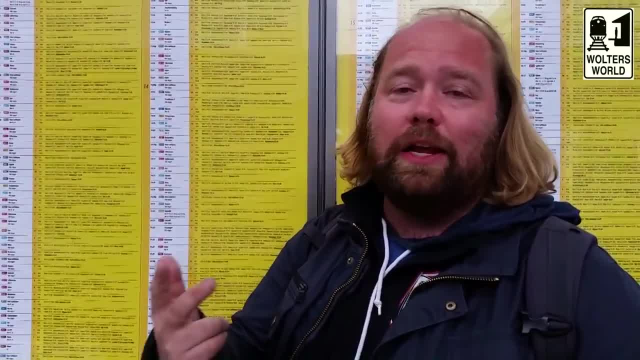 do the web one. If you're in the station going and you want to talk to somebody, get some help, you can do that. Use the kiosk and they're very simple in multiple languages all over Europe, So you can get an English, Italian, German anywhere in Europe. which? 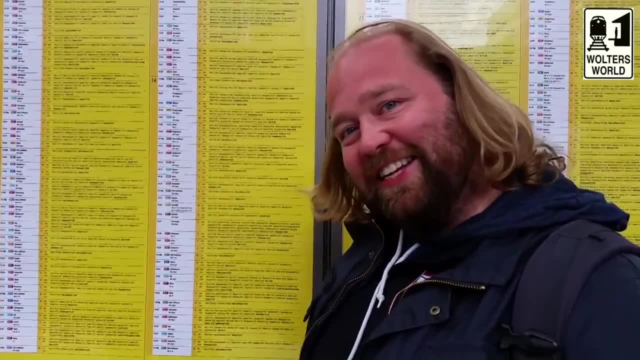 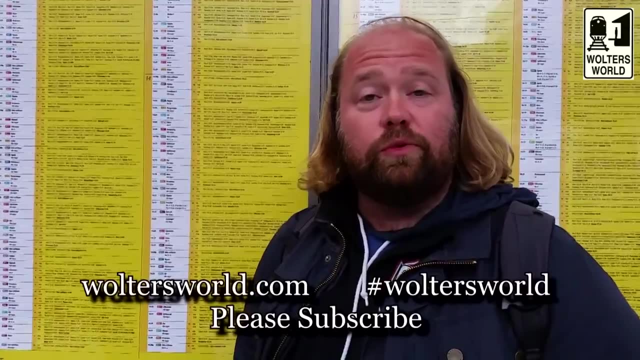 is really fantastic, And, of course, you've got the old-fashioned ones. I like to do like this. Anyway, if you want to learn more train travel tips or other travel tips, check us out on our website at waltersworldcom. We're also on Twitter and Facebook, and we really 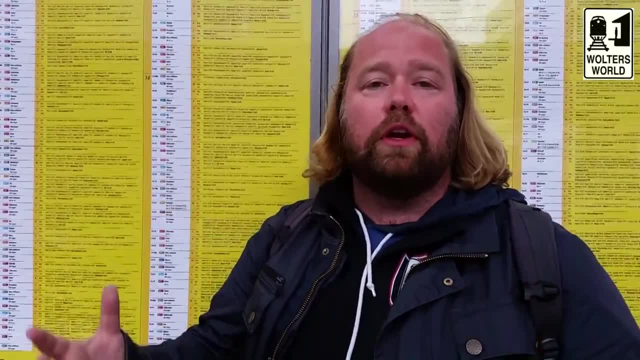 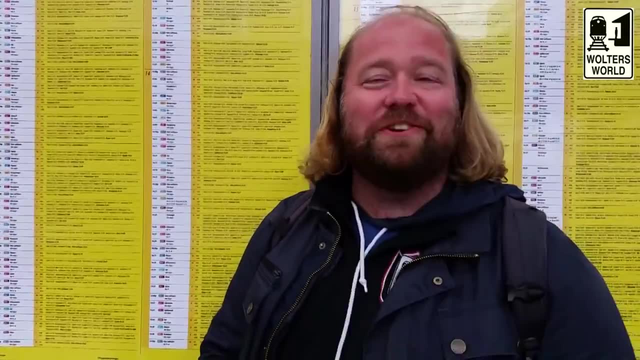 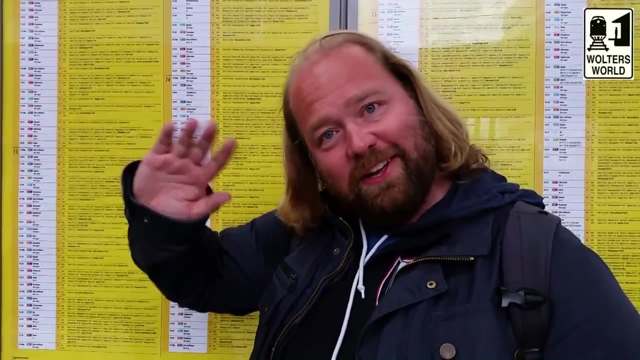 appreciate your likes and subscriptions, And if you love to travel like we do, we've got all kinds of videos, so please subscribe. And our newest travel videos: Five Things You'll Love and Hate About Oslo. Anyway, I'll say bye from here in Oslo, getting ready to get my train to Gothenburg. Bye.